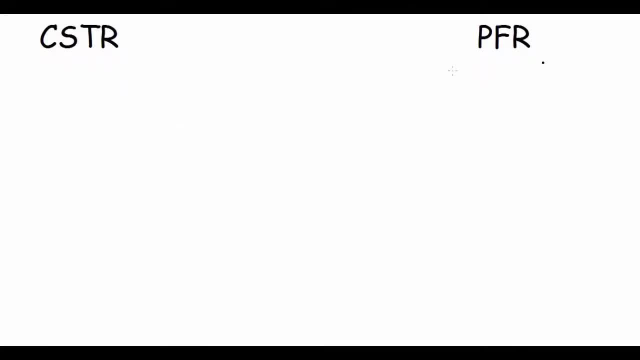 So let's discuss the differences between a CSTR and a PFR. So I will draw a line in between to make these differences more clear. So the first point under CSTR is so: CSTR stands for continuous stirred tank reactor- Let me underline this: Continuous stirred tank reactor- And for PFR- PFR stands for plug flow reactor, PFR stands for plug flow reactor. So now let's move on to the second point. 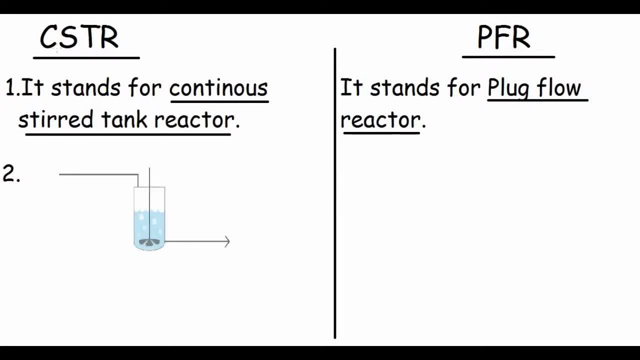 So this is a CSTR. This is the effluent stream. So this is the effluent stream and this is the input stream. This is the input stream, This is known as the agitator. So in this input feed, in this input, the kilomoles per hour of feed which is sent in is denoted by FA0.. FA0 is denoted by the molar flow rate, which is kilomoles per hour. 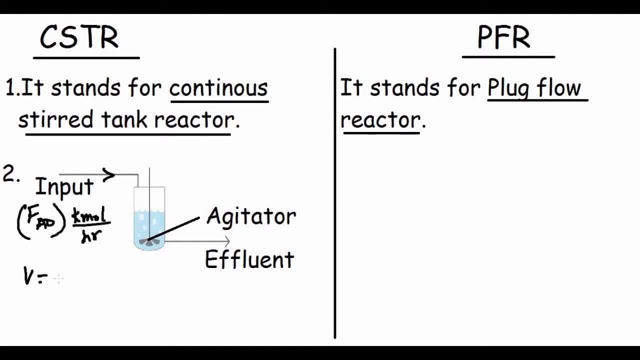 And the volume of F? pi is denoted by F. pi divided by M of this reactor is denoted by v. v is the volume of this reactor now using this parameter. using these two parameters, we can write the performance equation for this cstr, which will be shown in the 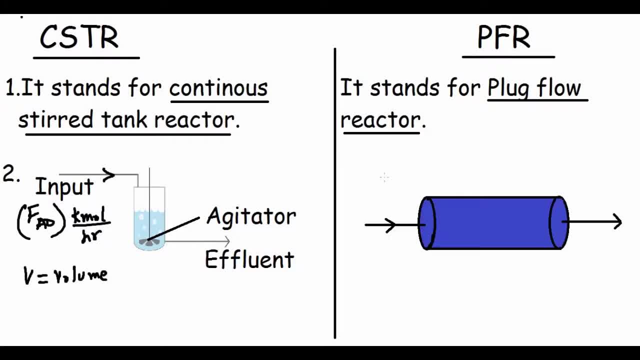 third point. now let's move on to the pfr. so this is what a pfr looks like. this is the input stream, this is the input stream and this is the effluent stream, or the output. so in order to understand plug flow reactor, first we need to understand what a plug flow is. so for that we will take a 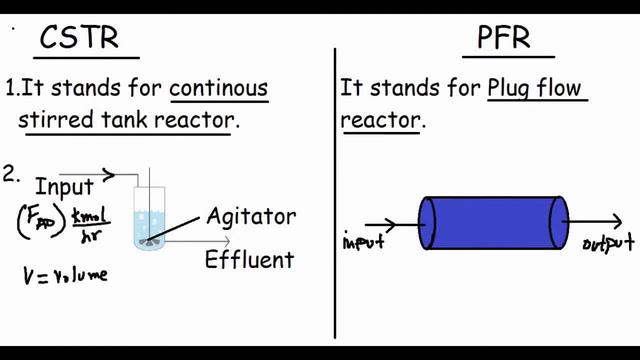 slice or an element from this reactor. so first we consider a laminar flow inside this a b c d region. a b c d region. so we consider a laminar flow inside this and let's look at the velocity profile of that flow. so for laminar flow, we all know that the velocity profile is parabolic and that is what 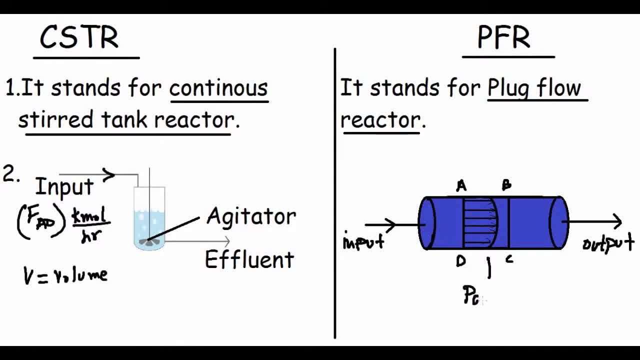 we see here. it is parabolic in nature. it is parabolic. now, what happens if we increase the reynolds number? if the reynolds number is increased further, then what we will see is this parabolic nature will start to flatten and it will look something like this. so you can clearly see that, as i have increased 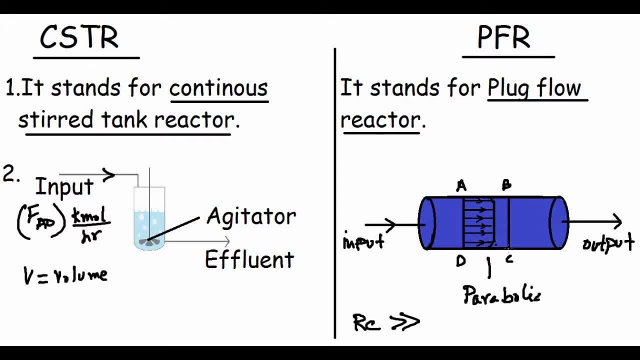 the reynolds number, these edges. these edges has started to become tappered and this has become a straight line. that is from a parabolic nature, that was for a laminar flow. it has started to become something like this, which is for a turbulent flow. 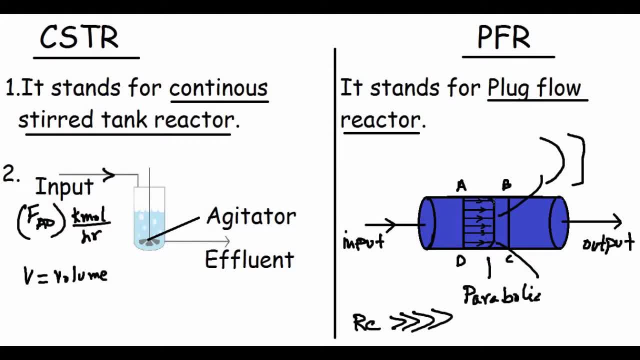 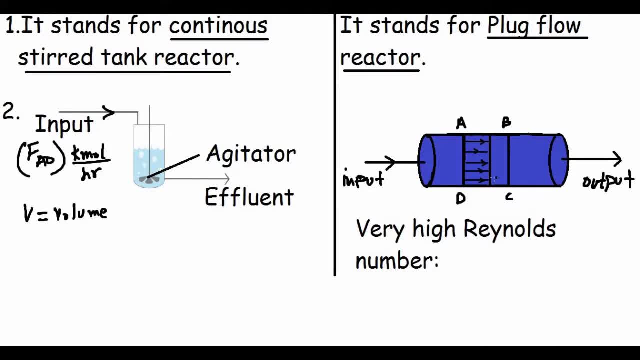 now, as you increase Reynolds number further, this entire thing will become a straight line. so for very high Reynolds number, this velocity profile has become a straight line. as you can see, this is known as a plug. this is known as a plug and hence the flow is known as plug flow, so a reactor in which these type of flow 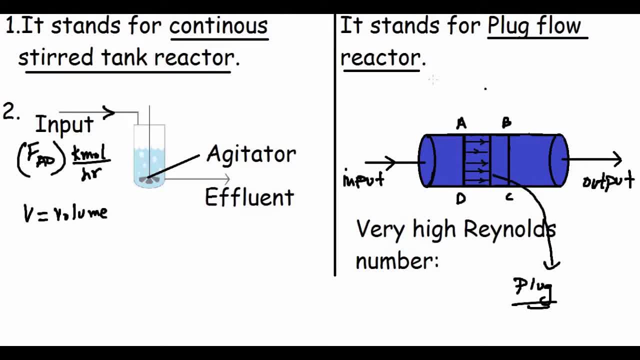 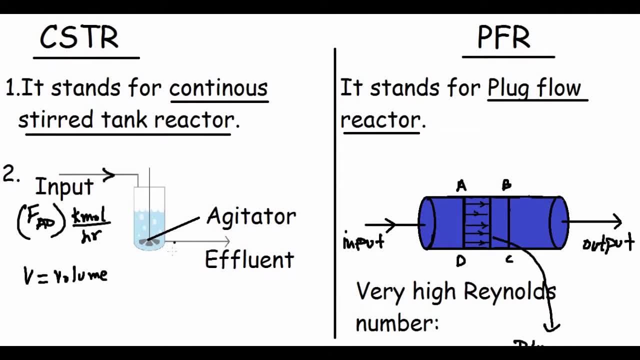 occurs or the fluid follows plug flow is known as a plug flow reactor. now the question is: how does mixing occurs in a plug flow? we can clearly see that in a CSTR, mixing occurred due to agitation. that is, agitator is fitted and its rotation or the rpm can be set, and likewise the mixing can be occurred. but 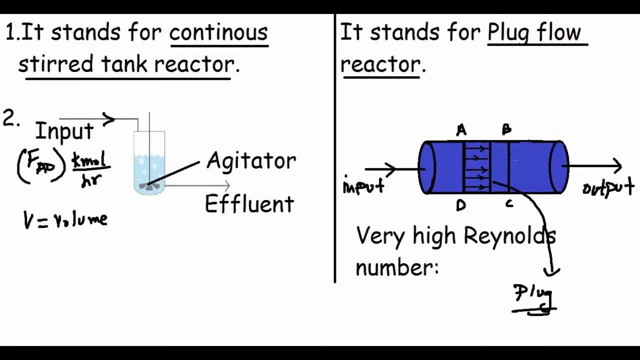 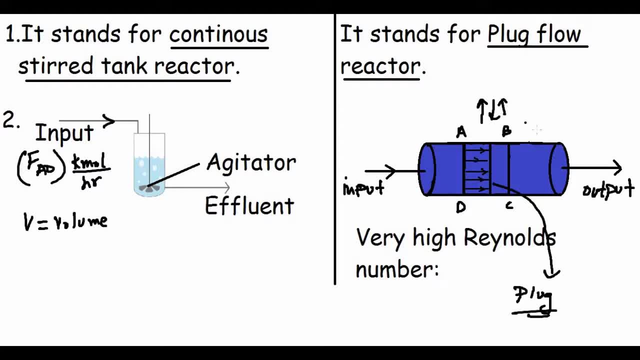 for PFR the mixing is somewhat unique. in PFR mixing occurs in the radial direction. mixing occurs in the radial direction and thus no mixing will occur in the axial direction. flow occur in the axial direction, but mixing within a plug occurs in the radial direction. so this: 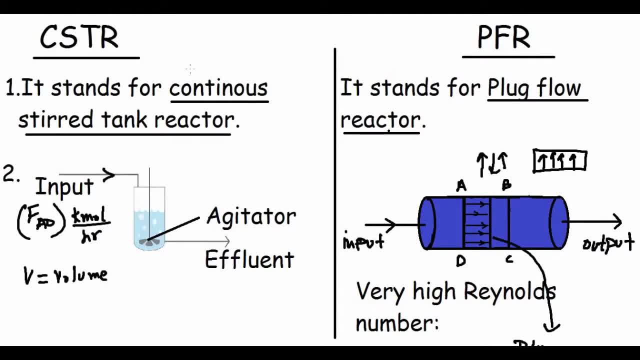 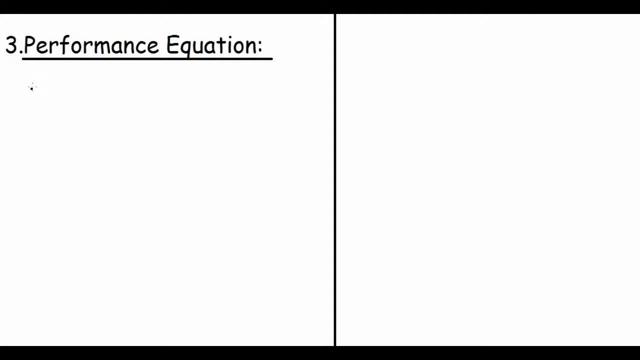 is a unique criteria for PFR. now comes the third difference. so the third point is the performance equation. for a CSTR, the performance equation is somewhat like this: V by FA0. V by FA0 is equal to XA by minus RA. so what does this mean? so in this equation, V stands for, V is the, V is the. 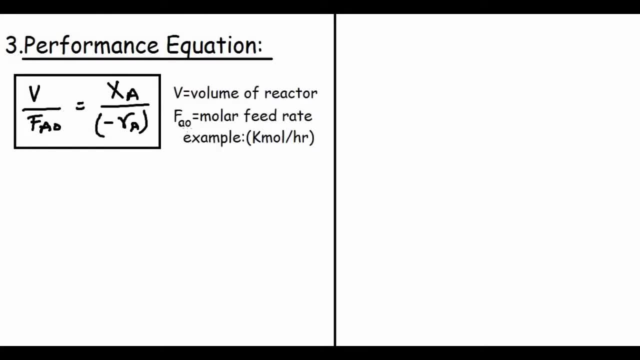 volume of the reactor FA0. FA0 is the molar feed rate. example of a FA0. units of FA0 is K moles per hour or it can be gram mole- gram mole per hour, something like that. that is the molar feed rate. so why am i writing FA0 and 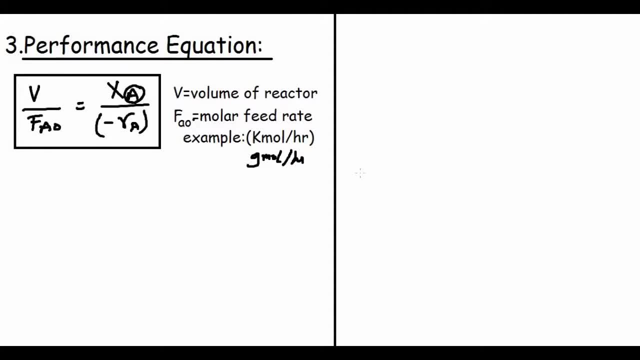 XA over here. what is the meaning of this A? so the reaction which we will assume is A giving R, A giving R, and it will be a liquid phase reaction. liquid phase reaction, so it is constant volume, constant volume. so that is what we have assumed and hence we are writing this. 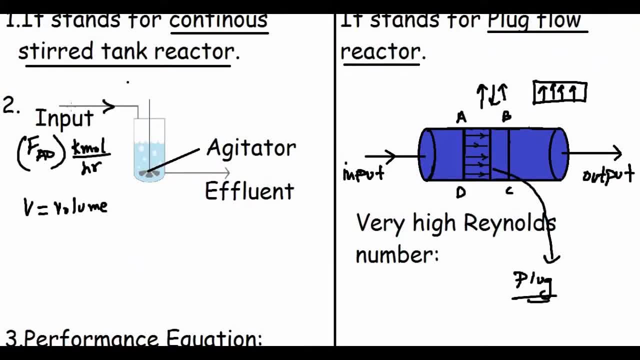 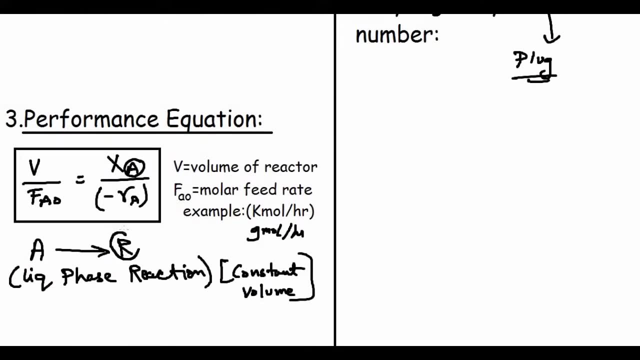 FA0 because the input, the input to this reactor, are FA, that is, A is the input in both of these. A is the input in the effluent stream. there may be some A and there will be R, because A is getting converted to R, so the conversion is. 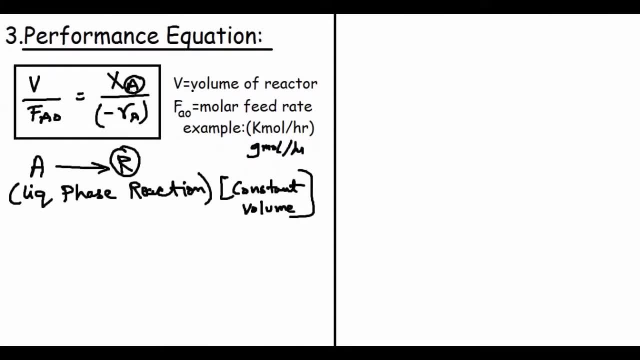 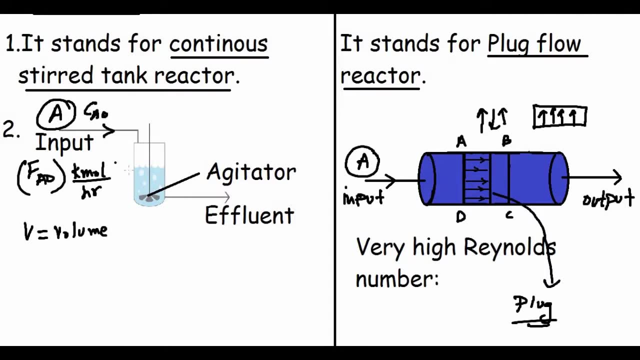 denoted by XA. now we will talk about this conversion. that is XA. so XA is given by 1 minus CA, by CA0. so what is this CA and CA0? well, when the input is fit, the concentration of A in this input is assumed to be CA0, and 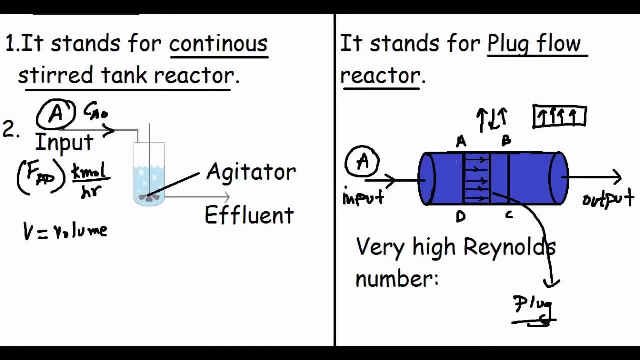 within the reactor, conversion will occur, that is, A will be getting converted to R. according to this reaction, A will be getting converted to R and hence the concentration of A will start to decrease. and within the reactor it is assumed that the concentration has become CA, so hence the conversion that 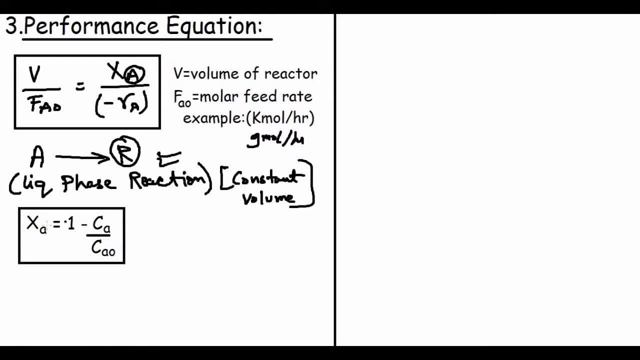 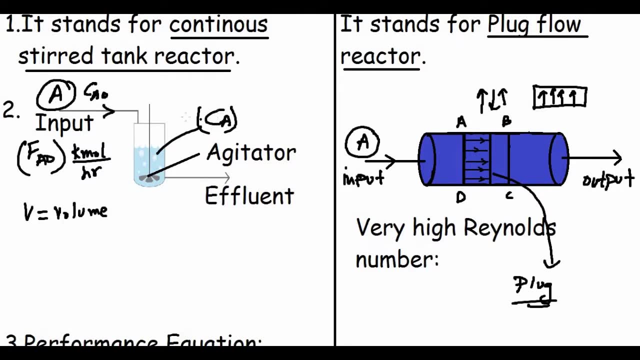 is the amount of A converted to R is denoted by XA and it is given by 1, minus CA by CA0. so you can check for one thing: that at the beginning, at the beginning, when the reaction was about to start, then CA, CA was equal to, CA was equal to. 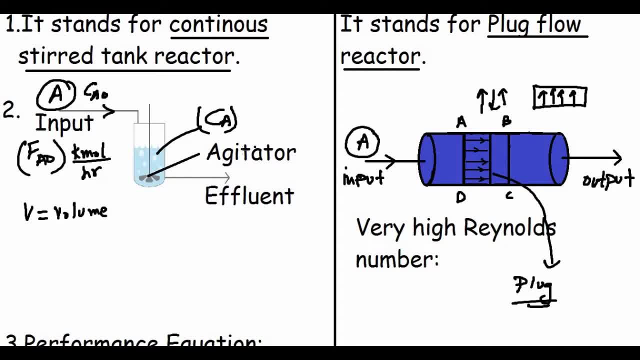 CA0 because at the starting, assume that the agitator has not started to work or it is at time- equals to 0, hence, at time equals to 0, CA will be equal to CA0, but as time progresses, the reaction will start to occur and hence this CA. 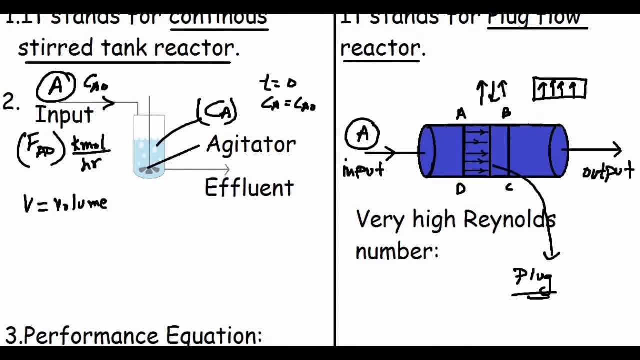 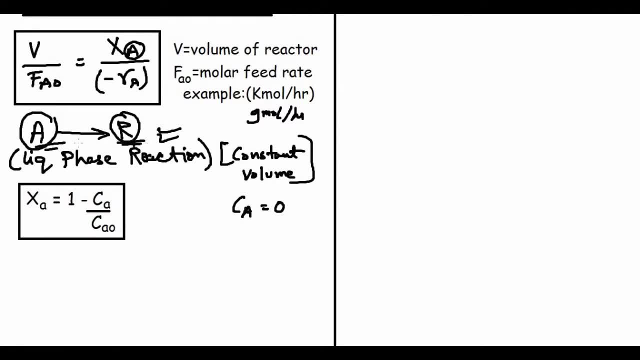 will start to diminish and if total conversion is achieved, then CA will become 0. CA will become 0 because entire A has been converted into R, so the concentration of A falls to 0 and this conversion, this conversion will become 100%. you can clearly see that CA equals to 0 implies XA equals to 1, which is: 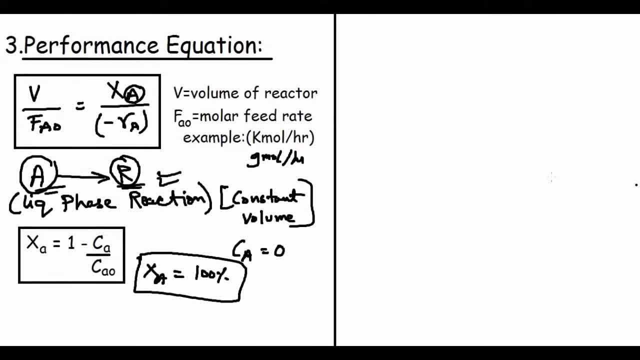 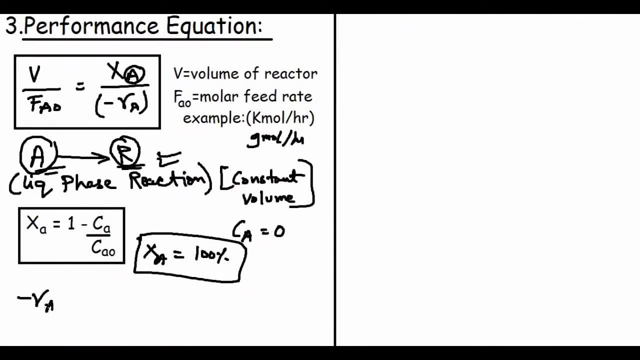 100%. so this was the performance equation of CSTR. now comes the minus RA part. this is basically the rate equation. for first order we write it as minus RA equals to K CA to the power 1. for first order we write: minus RA equals to K CA to the power 1, so 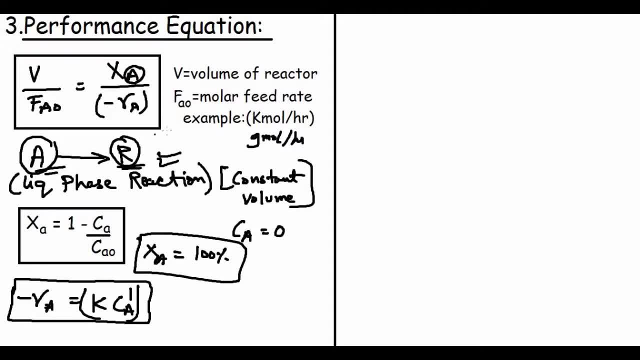 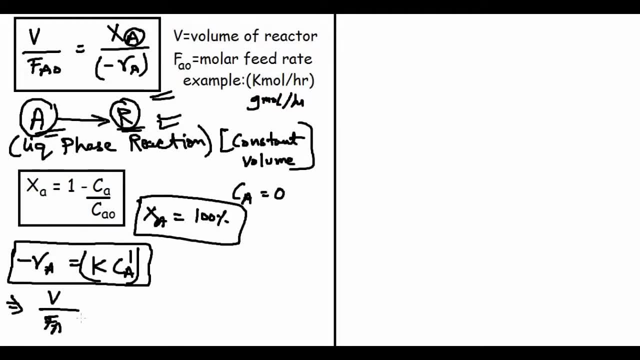 this entire thing is substituted in this equation and what we obtain is we obtain something like this: V by FA0 is equal to XA by K CA. so another thing: CA can be written as CA0. that is the initial amount minus XA by K CA. so this is the initial amount minus XA by K CA. so another thing: CA can be written as CA0. that is the initial. 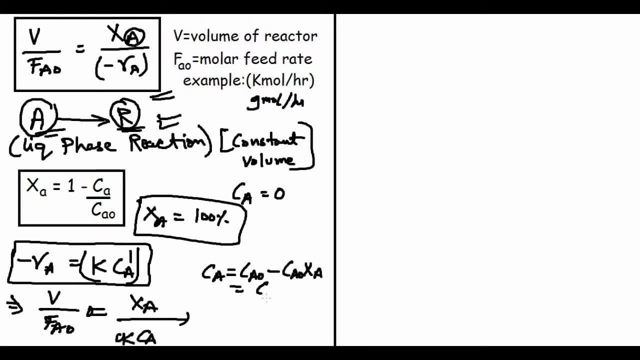 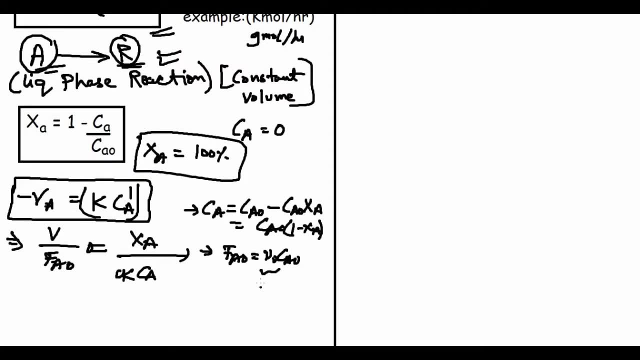 ca0- xa. that is the amount broken. so this can be simplified into ca0, 1 minus xa. and also fa0 can be written as: fa0 can be written as v0 times ca0, where v0 is the volumetric flow rate, that is, meter cubes per second, and ca0 is the concentration, which is k moles per liter. so you 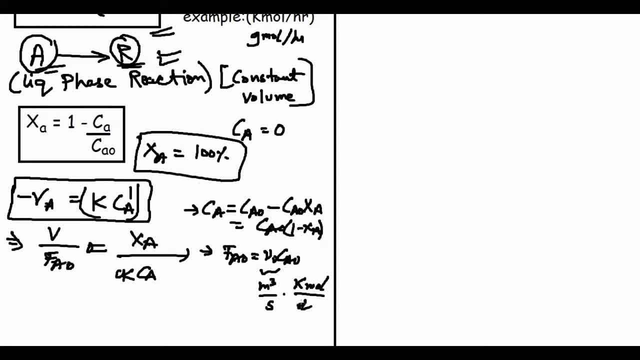 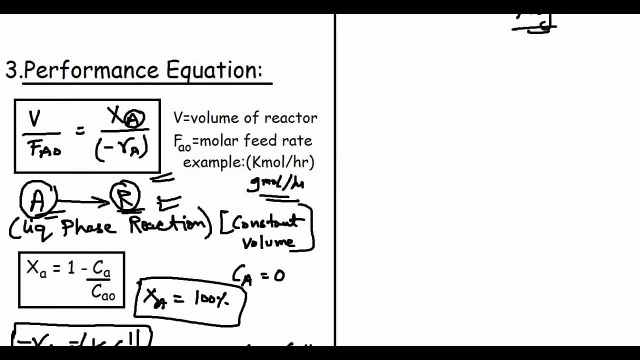 can see k moles per liter or k moles per meter cube, as i have taken meter cube over here, so i will take meter cube in ca0 also, so this will get canceled. and fa0 unit is k moles per second, which is consistent with our dimensions, which we have mentioned before, so hence we use these equations. 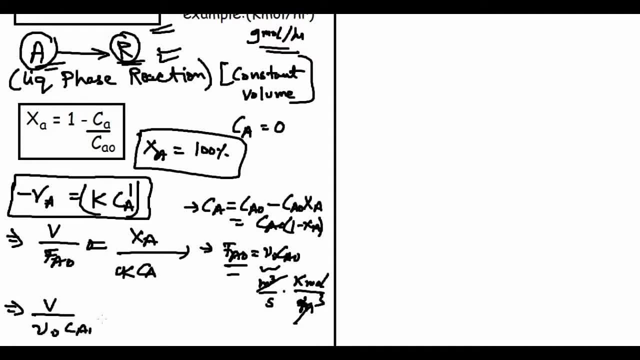 or we use these to substitute. in this equation we get: xa will be xa, and kca to the power 1 can be written as kca to the power 1 divided by xa square times xa to the power 1 square times xa. C A will be written as C A 0, 1 minus X A. So in this equation C A 0 will be cancelled. 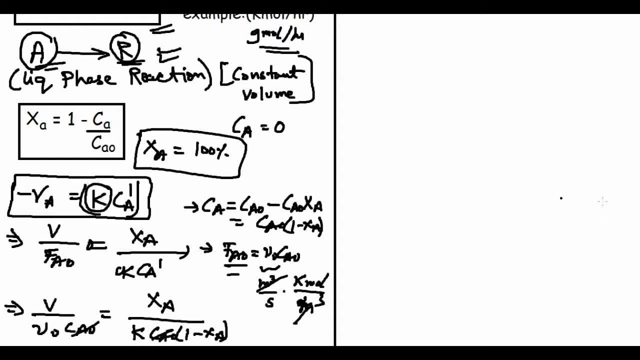 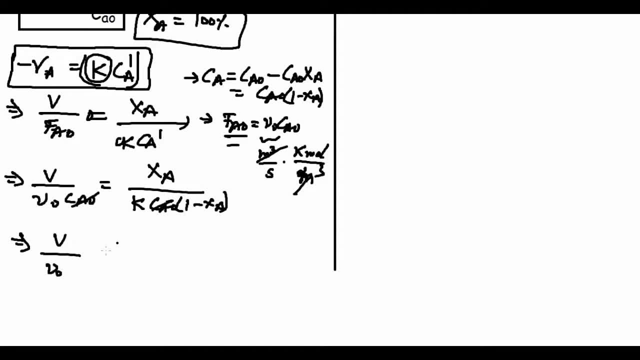 K is the reaction rate constant. K is the reaction rate constant. So now this equation can be further simplified into: V by V 0 times K is equals to X A by 1 minus X A. Now this V by V 0 has a special name, which is known as the tau. Tau is known as the space time. 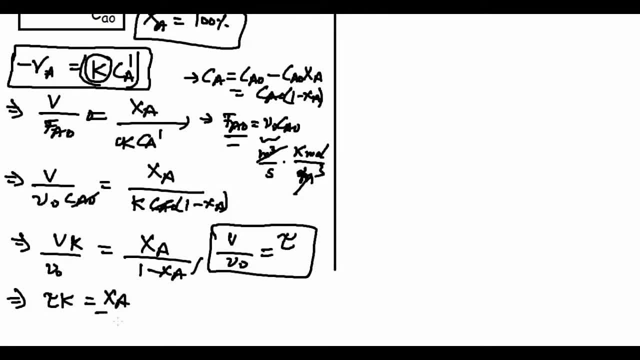 So we can write as: tau K equals to X A by 1 minus X A and the conversion. if we simplify this, we will achieve a conversion which is equal to tau K divided by 1 plus tau K. This is for a first order, CSTR. For a first order CSTR. 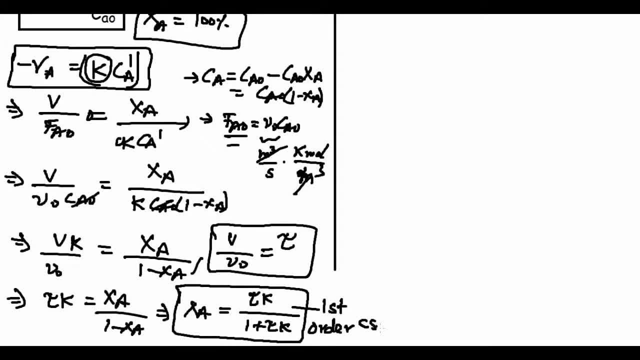 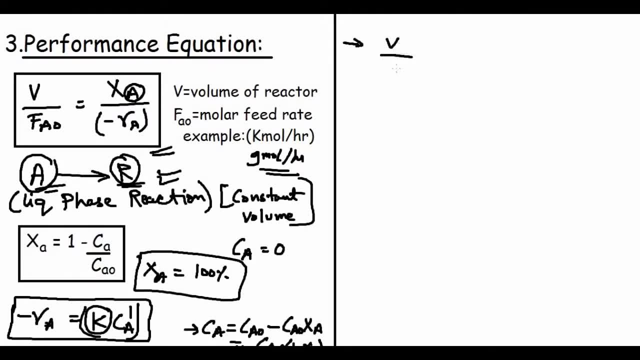 Now let's move on to the PFR. For PFR, the performance equation is a similar to the CSTR, but we have an integral. It is integral of D X A by minus R A. Now I have already explained the convention, So I am not going to explain it again. So we will write this: 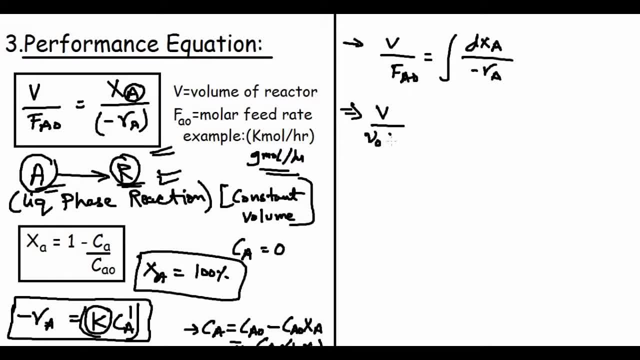 as F A 0, I will replace it by V 0 times C A 0 and integral D X A by 1 minus X A by 1 minus X A Again for first order. constant volume we have minus R A can be written as: 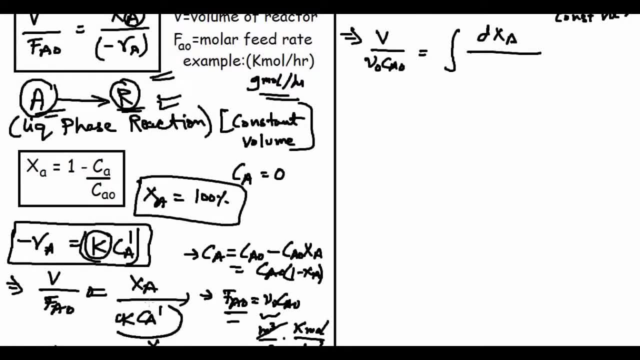 minus R A will be written as K C A to the power 1.. So here it will be K C A to the power 1.. This will be further simplified into D X A by K C A can be written as C A 0- 1. 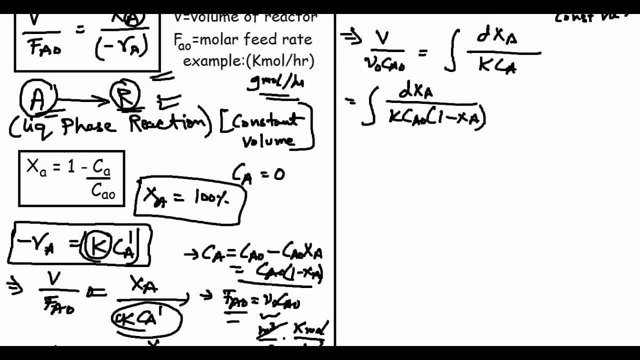 minus X A. So I have shown here why it is C A 0, 1 minus X A. So C A 0 will cancel from both sides and again what we will get is V by V, 0 is tau, So tau K is equal to this, K moves up. 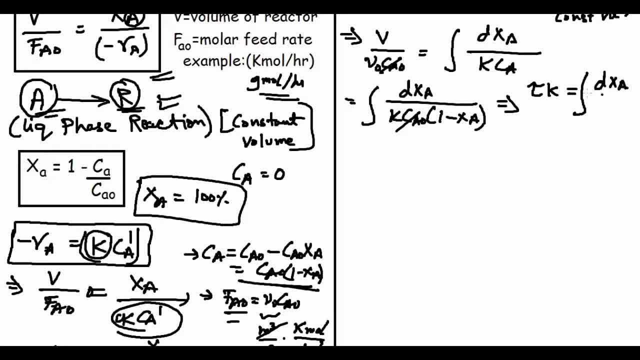 So tau K equals to integral D X A by 1 minus X A. So this can be written as: tau K equals to: let's take the integral from 0 to X A, from 0 to X A, because we are concerned with the expression. 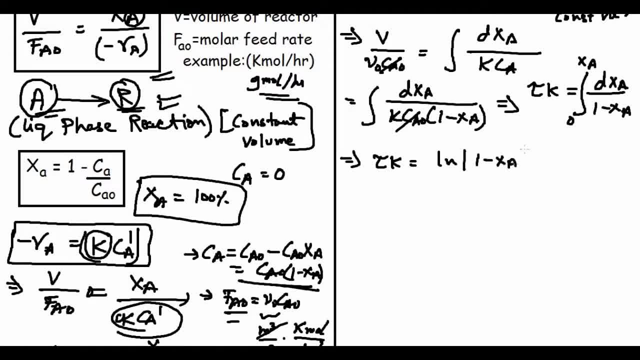 So this, on integrating, gives L N 1 minus X A, from 0 to X A and the negative will come out due to this negative sign. So minus tau K is equals to L N 1 minus X A minus L N 1. 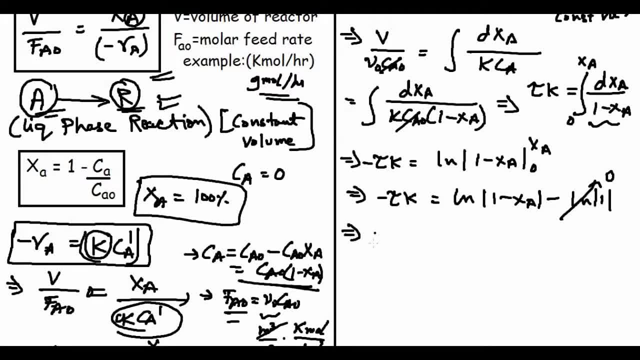 which is nothing but a 0. So this becomes L N. 1 minus X A equals to minus tau K, which ends up being 1 minus X A equals to E, to the power, minus tau K. So this becomes L N 1. 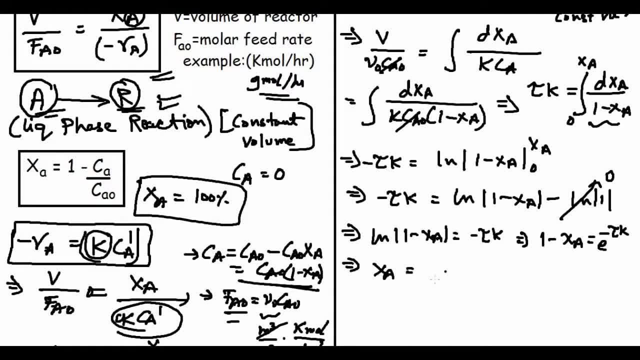 tau K and X A is equal to X. A is equal to 1 minus E to the power minus tau K. So this tau K has a special name. This is known as the D A, which is the dam collar number. This D A is equal to dam collar number, So D A is the dam collar number. So for both of this, 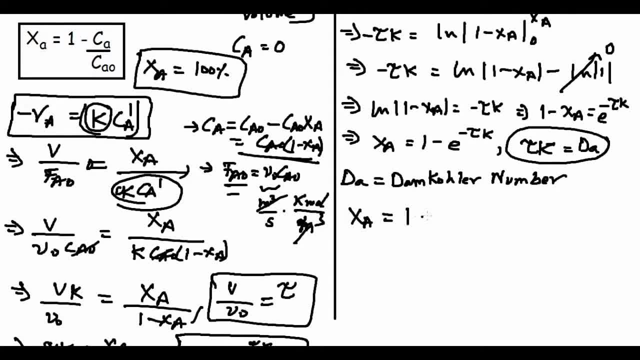 we can write The conversion. as for P F R, X A equals to 1 minus E, to the power minus dam collar number. This is for the P F R and for the C S T R, we can write: X A equals to dam collar number. 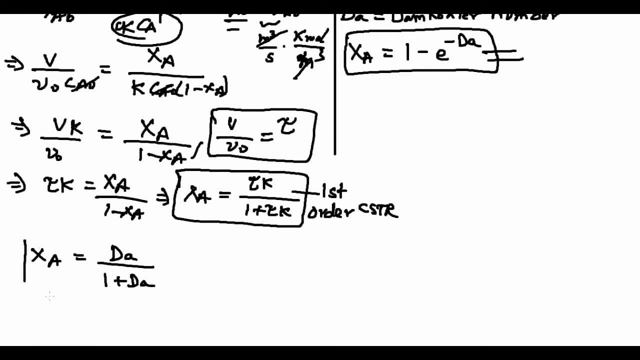 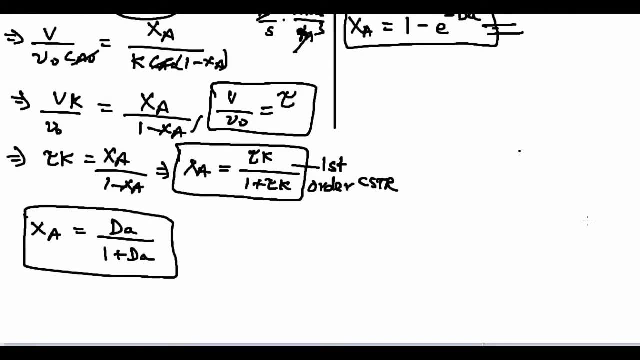 by 1 plus dam collar number. So this is for the C S T R and this is for the P F? R. Now the important point which I am going to write is that for same volume for same volume, So here we would write a positive order, say for, for C S T R, the conversion will be positive. 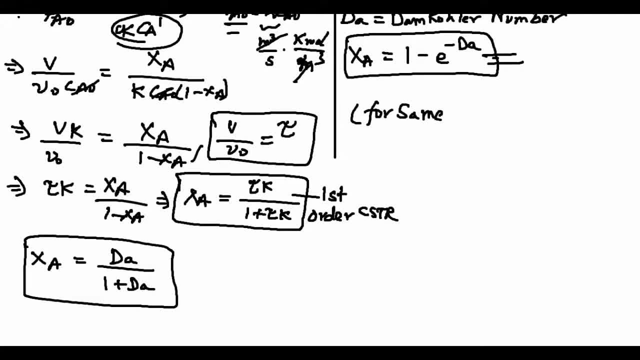 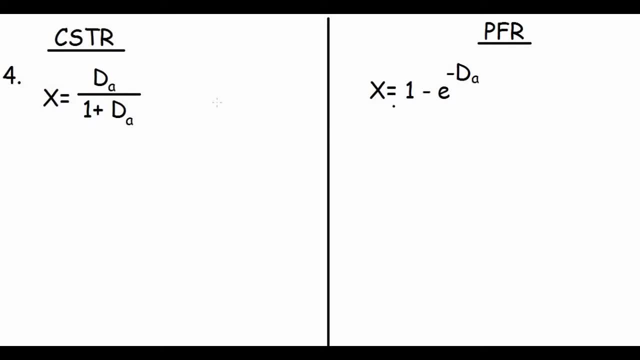 This will be the fourth point, So we have derived this expression in the previous slide and what we want to say is: for equal volume. for equal volume of C S T R and P F R, the conversation for a P F R is greater than that of the C S T R, So I will write this down. 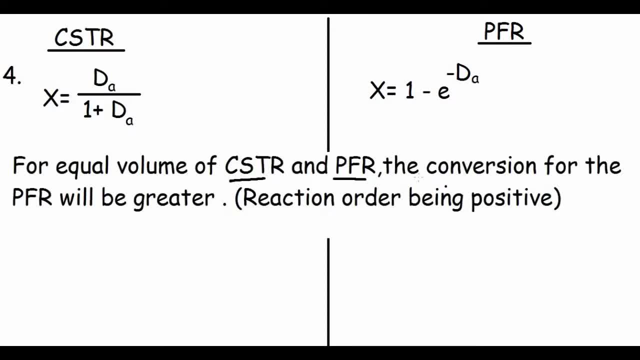 For equal volume of C S, T, R and P F R, the conversation for the P F R will be greater, reaction order being positive. So here we have derived these two for first order reaction, which is a positive order. So now, if you put values of Damkohler number, you will observe that for PFR the x will be greater compared to the CSTR. 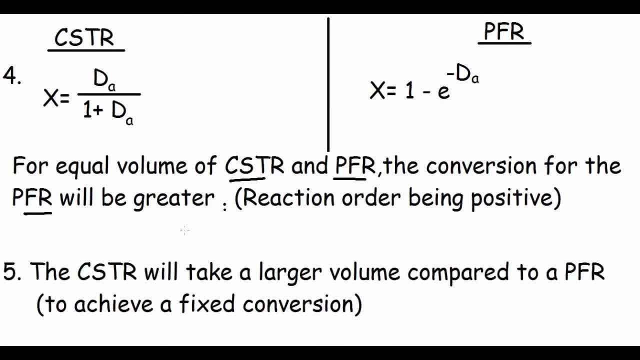 So let's move on to the fifth point now. So this fifth point says the CSTR will take a larger volume compared to a PFR in order to achieve a fixed conversion. Now, to explain this fifth point, I will require a graph and the performance equations of each of these. 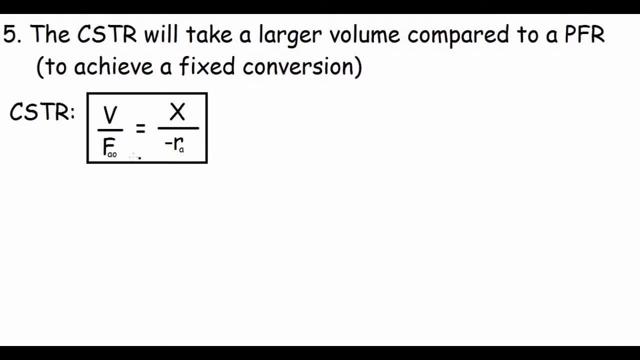 So let's write the performance equation first. So this is the performance equation of a CSTR: V by FA0 equals to x by minus RA. Now this V is the volume of the CSTR. So if we plot a graph, 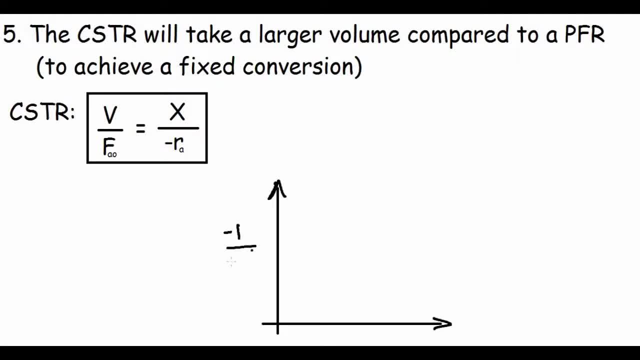 So we plot a graph for minus 1 by RA and xA. This is the conversion, So the graph looks somewhat like this. So this, So this graph can be obtained experimentally, and now suppose I want a conversion of 0.75.. 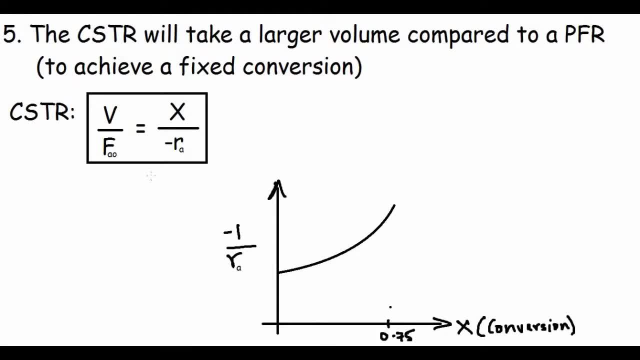 This is what I require. So, in order to find the volume, what I require is to find the area under this curve, that is, this area: ABCD, ABCD. This area, that is this rectangle ABCD area, will give me the x by minus RA, that is. 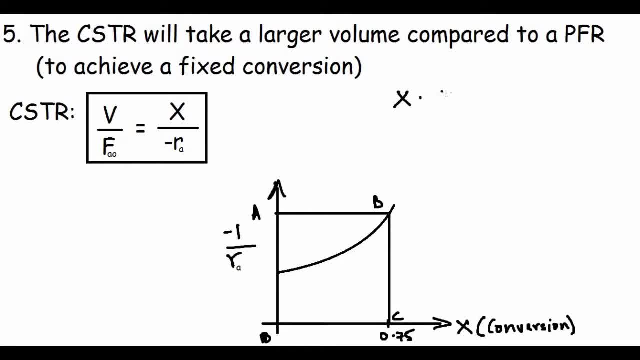 I am multiplying x with 1 by minus RA, So this entire thing is V by FA0.. So this entire area ABCD will give the V by FA0 term. Now FA0 is constant, So I can say that this volume of the CSTR is proportional to the area ABCD. 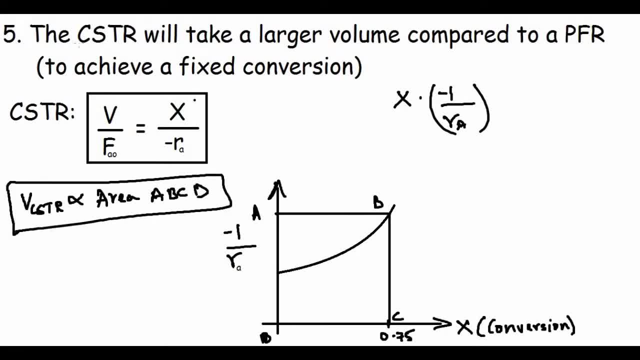 So this is the first step. Now let's move on to the PFR part. So for PFR the performance equation is: V by FA0 equals to integral 0 to xA, dx by minus RA. So this is the performance equation for PFR. 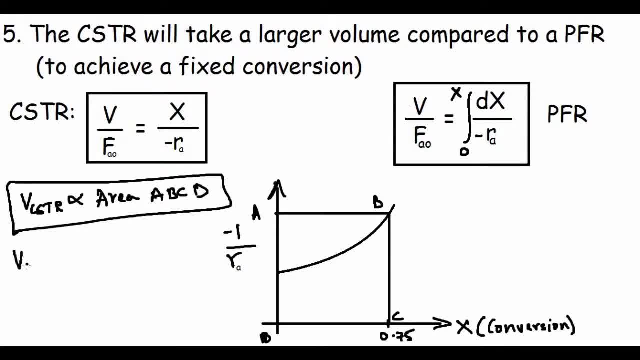 Now to find the V PFR, V PFR. This will be proportional to the area under this curve. So to find the area under this curve from 0 to 0.75.. It is simply this area shaded by this green color. 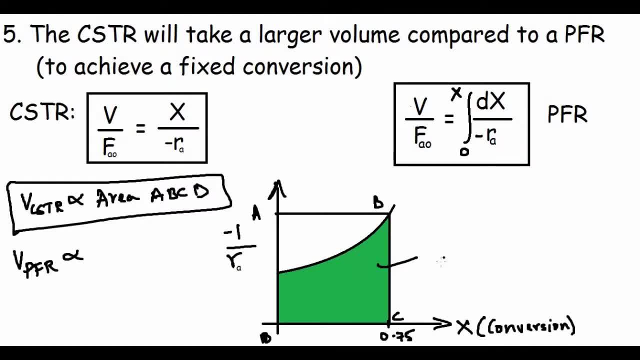 So this is the area which is for the PFR. So this is the area which is for the PFR. Let me name this area of, let me name this point as E, So this becomes BEDC, So it is proportional to area under BEDC.